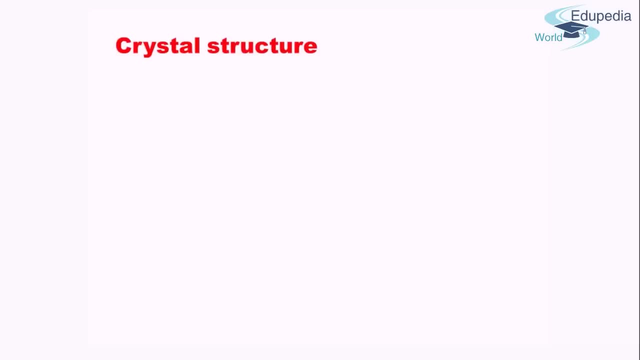 Let's go into details and understand what I am talking about. So, as I said, the properties of a material are influenced by a material, By its structure. how is the structure of a material helps define the end property of the material. Therefore, it is quite pivotal to understand and enhance our knowledge about the structure of a material. 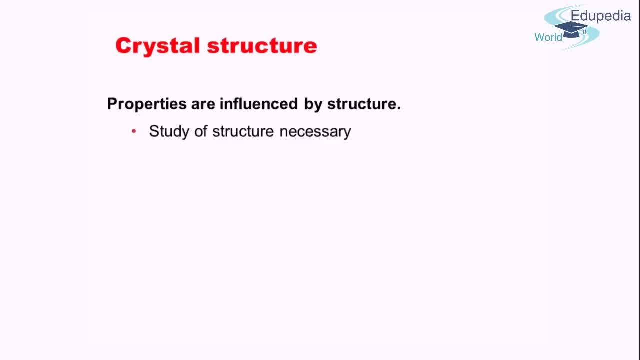 Now, broadly speaking, any material can be classified into two categories on the basis of structure. Right. So the solids exist as either a crystalline material or a monochromatic. So they are the material that is determined by the solid. But the solid or emmorphous materials. we will be focusing on solids because the abundant amount of elements and all the alloy systems are in the solid state. 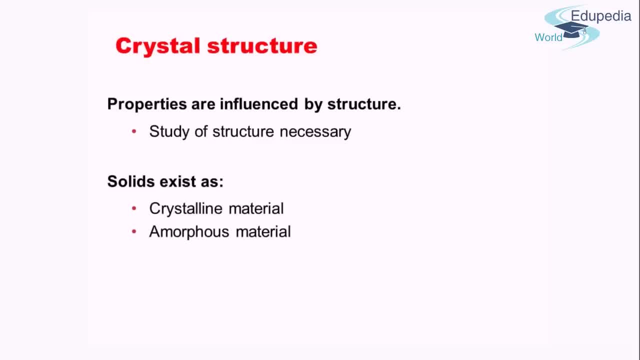 And most of the material science will deal with that, so we will focus on that for the time being. Now, what does each of them mean specifically? Solid exists as a crystalline material or amorphous material. Crystalline material means there is a long-range order in the material. 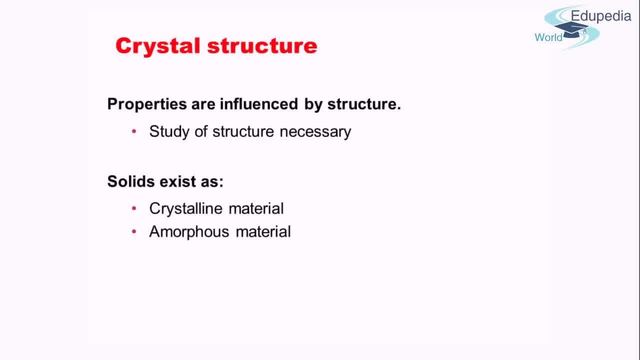 there is no ordering in the material. in the next slide we will discuss it further. let's see crystalline material, as I said, has long-range periodic arrangement of atoms. that is, if I give you if there is an atom here and here and the material is crystalline, then you can predict where will be the next atom. 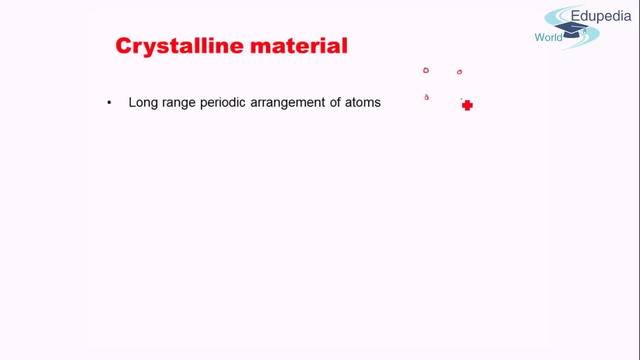 that is it is. it has a specific location where the atom can be present and there are locations where atom cannot be present. that is what is meant by long-range ordering. right now, this long-range ordering is a repetitive 3d pattern, that is, the ordering is present in the three dimension, so it will be in. 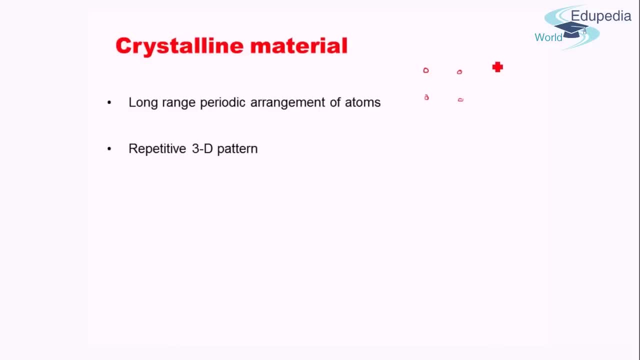 x-axis, y-axis and z-axis. there will be ordering in this direction, this direction and this direction, and that is typical characteristic. a 3d pattern is a typical characteristic of a crystalline material. now, as i said, there is a pattern in a crystalline material. you might ask: 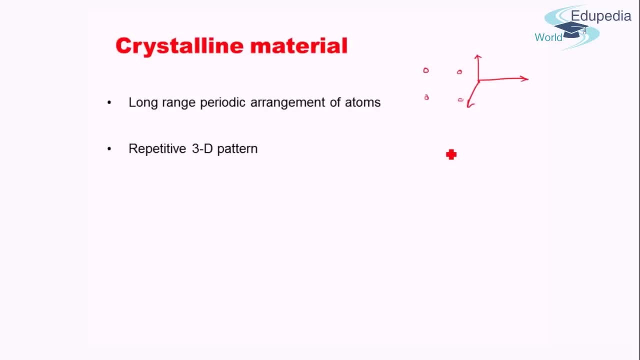 that there must be a very basic unit in the three dimension that can be repeated over and over again to get the whole 3d, isn't it exactly that is how it happens. there are what is known as unit cells. we'll come into that. those unit cell is the smallest block of 3d space which can be repeated. 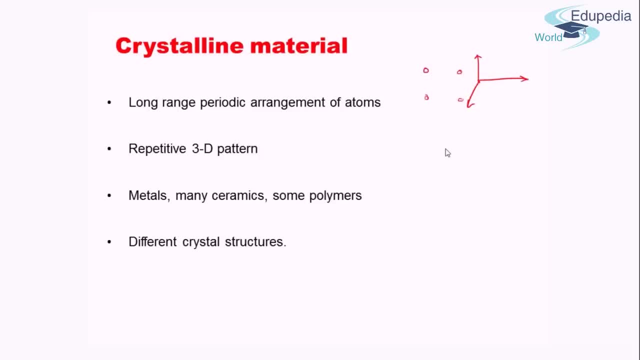 in x-axis, y-axis and z-axis to give you the whole 3d pattern of the crystalline material. therefore it is called the unit cell. it's the very basic building block of the crystalline material and that's why it is called the unit cell. 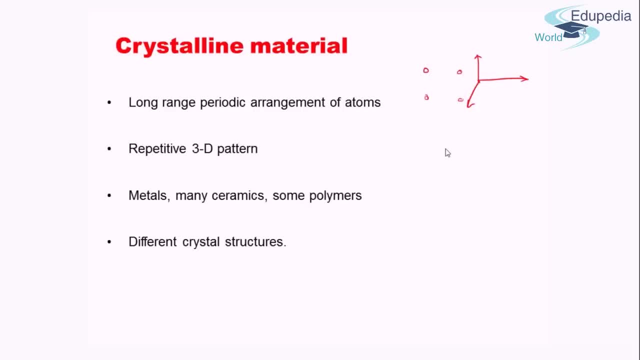 it's the very basic building block of the crystalline material and that's why it is called the unit cell crystalline material. now, to put things into perspective, crystalline material composes of most of the metals, a lot of ceramics and some polymers. when I say metals, I include metal as 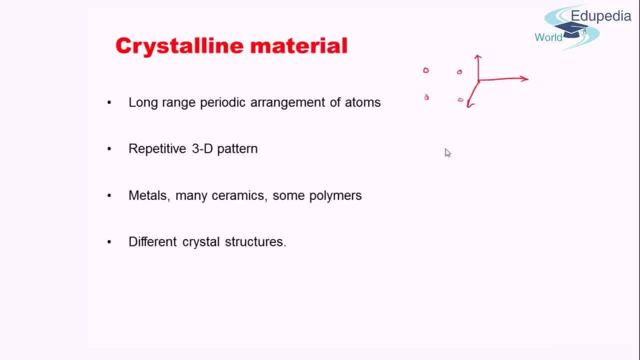 in elemental metal as well as alloys, which has combination of different metals. okay, now you can say that, okay, it's all fine that we have 3d arrangement, but is it possible to have different kind of 3d arrangement? actually, as it happens, there is a possibility to have different. 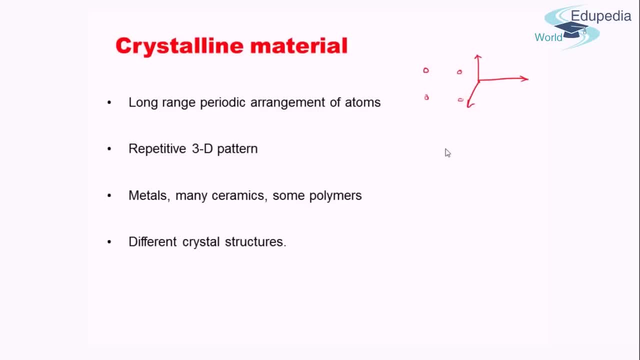 kinds of 3d arrangement. but the different kind of 3d arrangement can be grouped into seven crystal system and further classified into 14 Bravais lattice, so that 14 Bravais lattice kind of includes all the possible 3d arrangements that can be present in the crystal system. so that's. 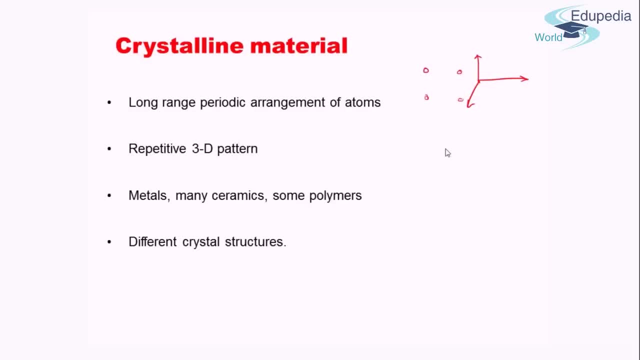 why it is called the unit cell. it's the unit cell that is present in a crystalline material, will not go into the 14 Bravais lattice will see the seven crystal systems. that's what I have written here, that there are different crystal structure need not be one type of 3d arrangement and the 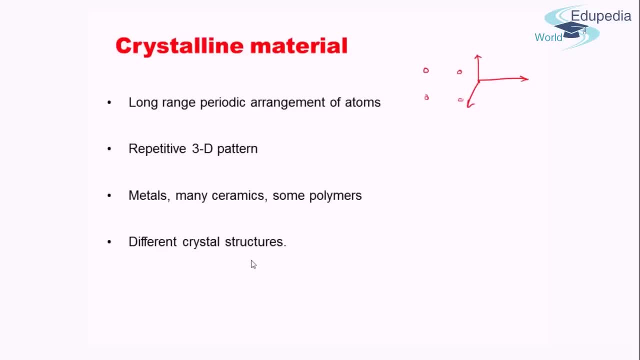 different crystal structure has a lot of influence on the property. that kind of determines a lot of property the material will have. so it is quite important to understand what category of crystal, trickle or a metal come under. now we have seen what is the crystalline material. alternatively, what? 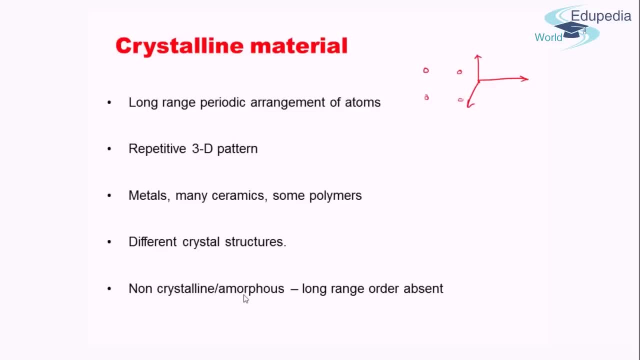 is a non crystalline or amorphous material. this both are alternative caves for the same thing. those are materials which do not have a long-range ordering. what do I mean? long-range ordering? I have written long range ordering here and long-range order here. so if there can be short-range ordering, 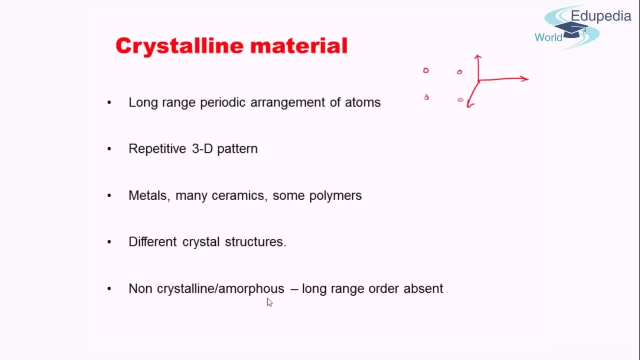 like there can be order in a material which does not have a short range ordering, which is long range ordering material, let's say in 10 atom length or 100 atoms length, but it does not extend throughout the material right or to a large macroscopic region. long range order is absent in such 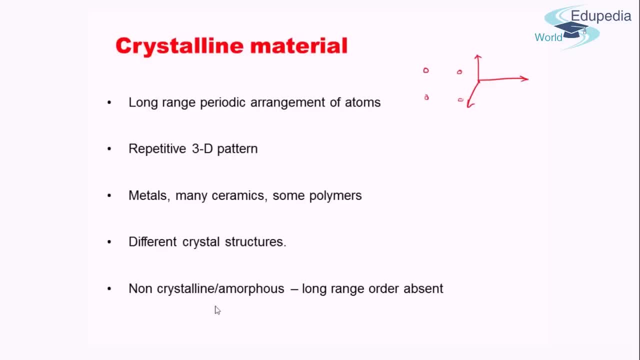 a scenario, and that scenario will result in a non amorphous material. a very simple example of non amorphous material which you all have seen is silica or sand. it is a non amorphous material though the silicon has kind of a sp3 hybridization. it should have three bonds. 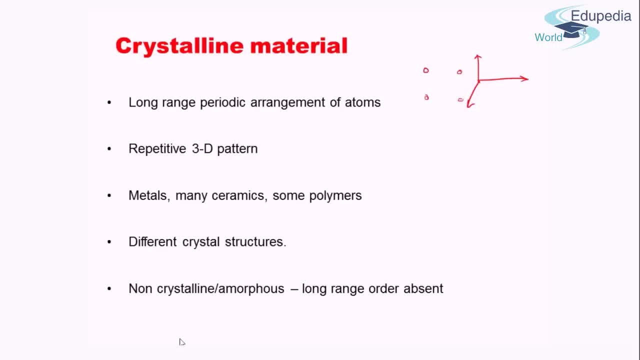 attached to it but it does not have. there are many broken bonds. as a result, the 3d repetition does not happen, as it should happen. thereby, it is amorphous. okay, now that we have got a glimpse into what is a crystalline system and what is an amorphous material, what is? 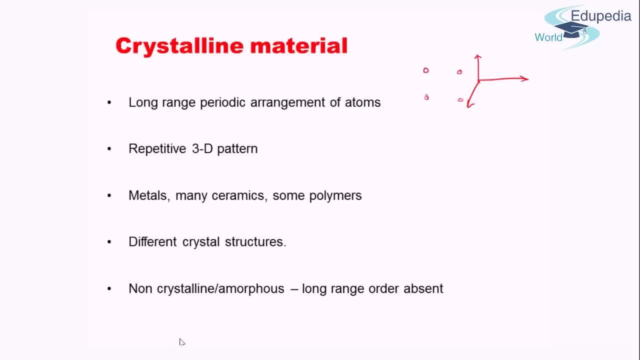 an amorphous system. let us dive deep and understand the different kind of crystal structures that i have mentioned here. okay, before that, let's discuss some more thing. the metal system that we will be discussing throughout our lectures will be based on hard sphere model. now, what is hard sphere model? hard sphere model assumes atoms to be like. 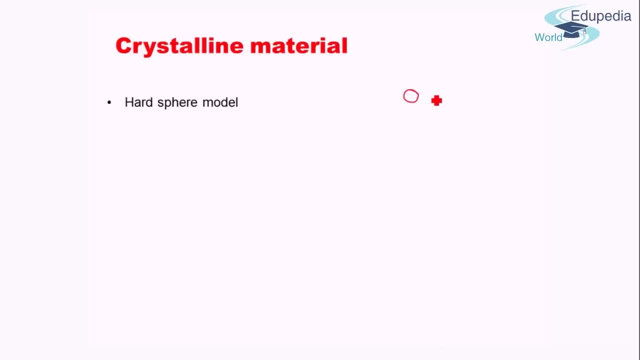 marbles, hard marbles. if there is one atom here, then another atom is here and this cannot intrude into the space here like there is a physical repulsion. these are. this is hard sphere. model atoms are considered hard spheres. unit cell, as i already discussed, is the smallest building block which can be repeated in the three dimension to get the 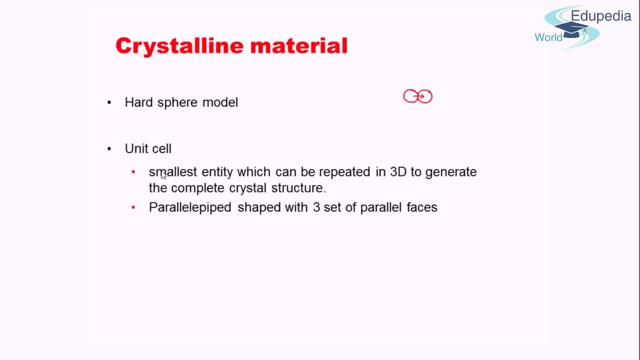 whole crystalline material, now a unit cell. what is the characteristic of a unit cell? a characteristic of a unit cell will be that it will have three dimension. it will have a x, y and a z dimension. and it might be something like this, like a cube which this angles as 90 degree and all the sides equal. 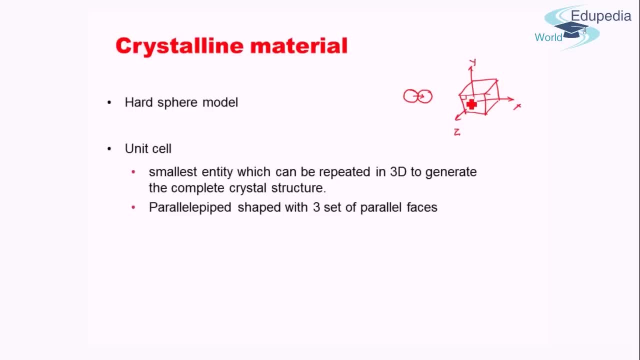 or it might be a cuboid which all with all the angles as 90 degree but the sides not equal, and it can take other configurations too that we'll see in the next slide. but to give you an idea, unit cell is composed of three set of parallel phases. this phase and this phase is parallel to each. 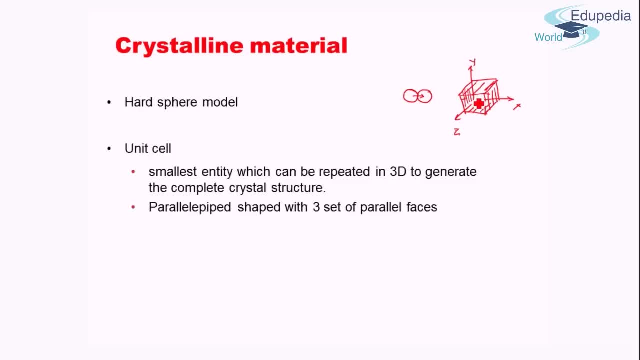 other. this phase and this phase is parallel to each other, and the front phase and the back phase are parallel to each other. so it is a parallel pipe shaped with three set of parallel phases. as i said, there are seven crystal systems and there are 14 types of. 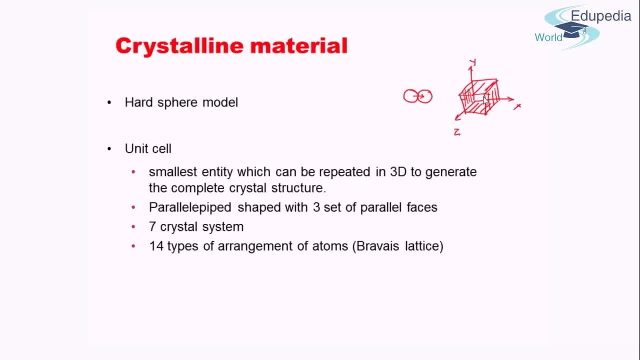 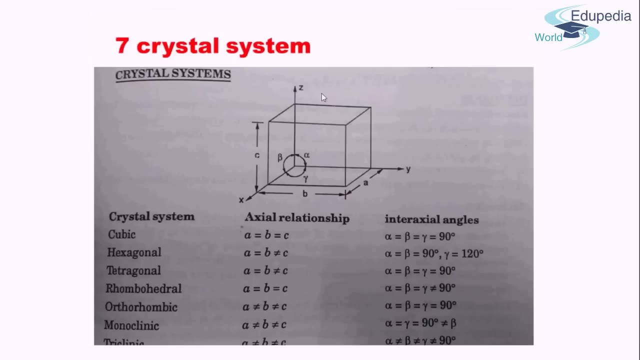 arrangement of atoms that can take place in the seven crystal system. so total of seven bravais 14, kind of arrangement, known as 14 bravais lattice, exist fine, so now let us see what are the seven crystal systems. this is the unit cell which i have shown over here. 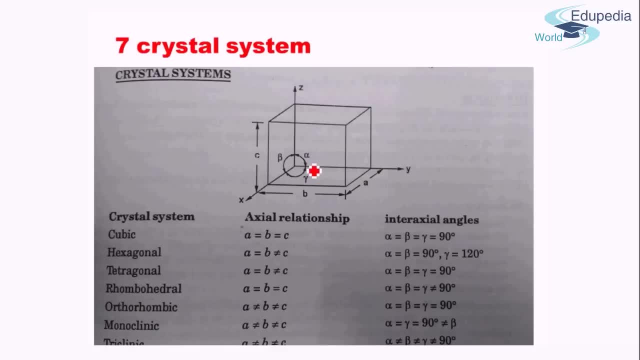 but the only difference being this: angles are alpha, beta, gamma and the lengths are in the x-axis. here they have considered this as the x-axis a, this is the y-axis, so they have the length is b and this is the z-axis and the length is c. okay, so these are the. 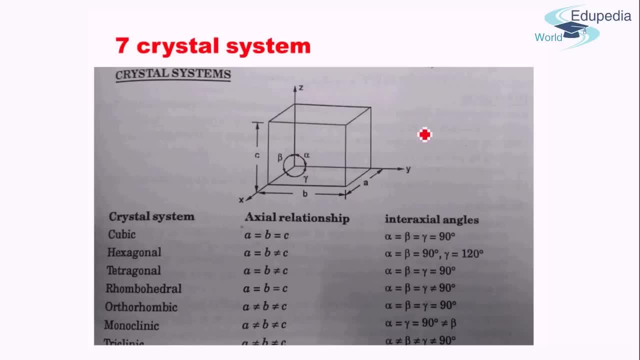 six variables which define a crystal system: the angles alpha, beta, gamma and the sides a, b, c. now the different combination of angles and sides will give rise to seven different kind of crystal system. let us see each of them one by one. the cubic system, which will be the most. 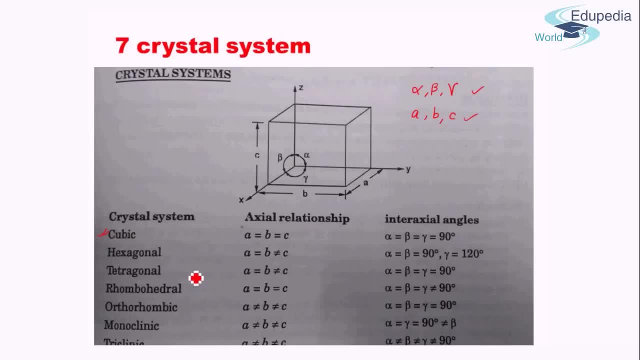 popular system in the metal system scenario, which, day in and day out, is the cubic system and that has all the three sides of equal length and all the three angles, 90 degree, okay, second, the hexagonal system. this is the second most important crystal system. when we talk about metals, in hexagonal system, we have two equal sides and a different third. 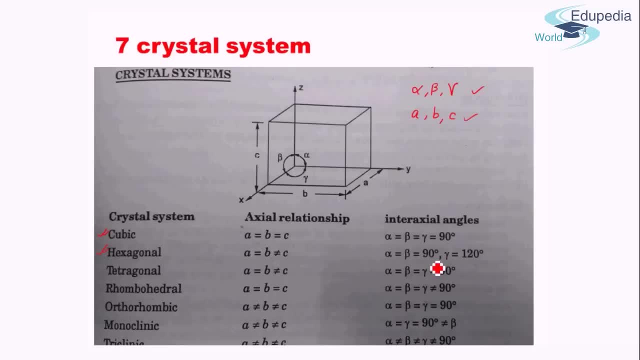 side and two angles as 90 degree and the third angle exactly 120 degree. for a hexagonal system which do not has have any stress inside it, c is approximately equal to one point, six, three, three times a, but you need not remember this. the basic idea is two sides are equal. 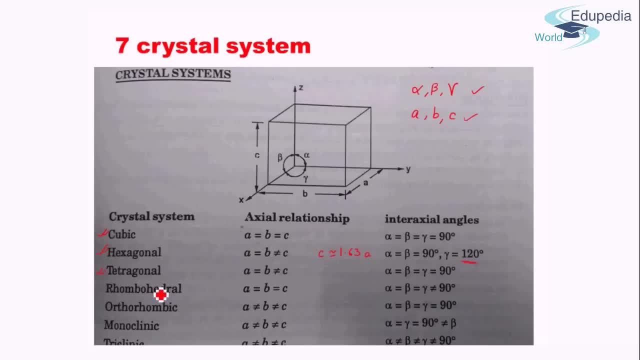 third is not equal tetragonal. you can think of this as a, not exactly a match box, but some thing which has two phases of the equivalent. this is a square, an almost like a square, but the third time its own was, to a very large rate, j место. whatever we see here is a is. 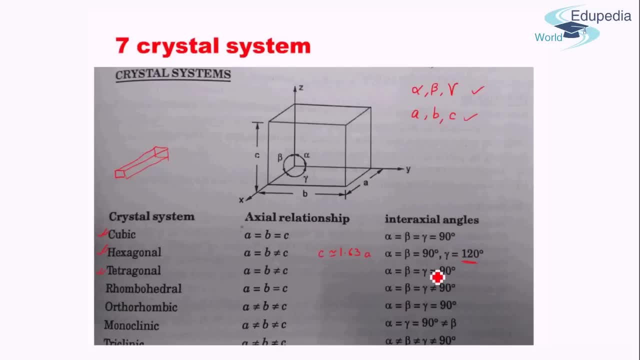 going to be what she's different and all the three angles are intended. thing break soon, that is that hater rumpo, heầner in is three angled c rooms, side c weather. the three angles did not go all equal, admit. different from ninety, do the part there is still three handled. 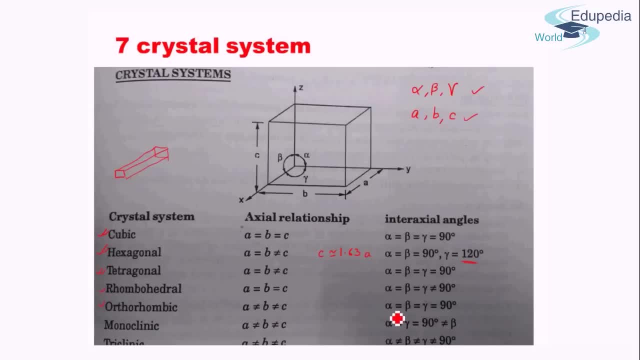 is good. no side equal, but all the angles equal to 90 degree. monoclinic has no side equal, two angles equal to 90 degree and the third angle is not equal to 90 degree. and finally comes triclinic. this is the most non-symmetric system in which none of the angle is equal. 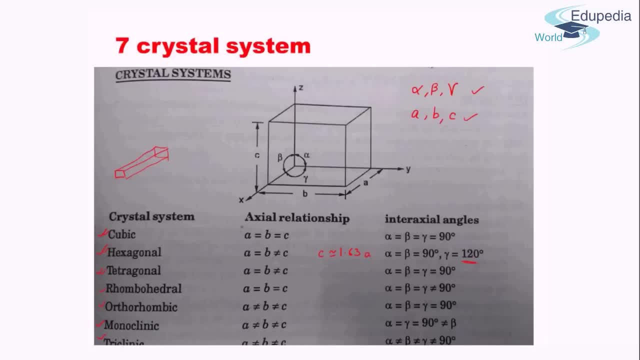 rather, none of the sides are equal and none of the angles are equal to each other and none of the angle is equal to 90 degree right. so we see that these are seven different kind of systems which can exist and based on which all unit cells can be defined. 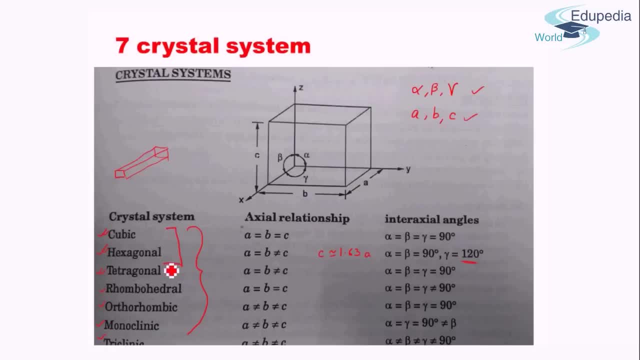 but as i already mentioned this, two- the first two will be the most important for our course and in fact even in advanced courses, when we focus mainly on metals and metal alloy systems. cubic and hexagonal are the most important systems. now there are four different ways in which atoms 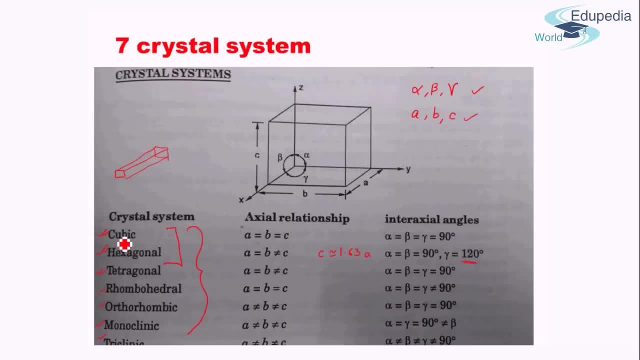 can be arranged in a system, right? this basically gives you just the outline of the unit cell, but this does not tell you where the atoms are going to be placed. so what are the four different locations where atom can be placed? those are: one is simple. I will take the example. 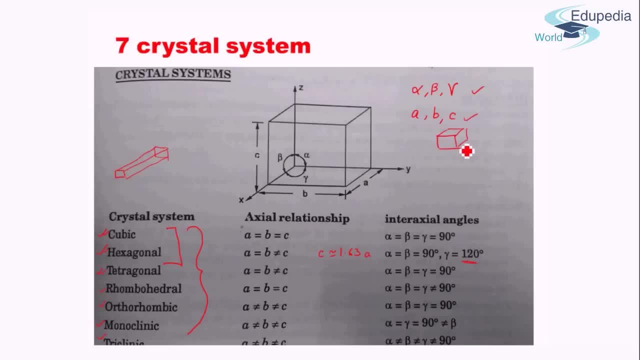 of cubic system. let's say, in the simple cubic system, only atoms are occupied at the eight corners. okay, this is simple. okay. second system is known as the body-centered. in body centered, what happens? in addition to the eight atoms at the eight corners, we have another atom. 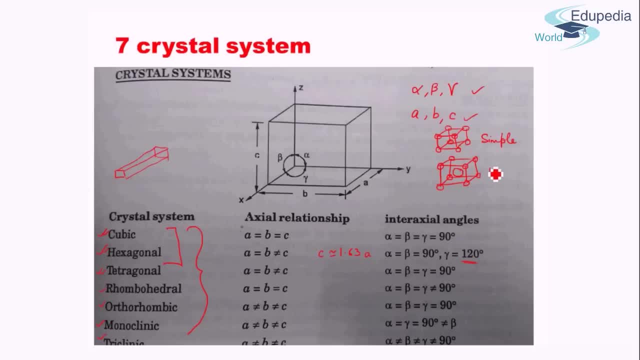 at the center. right, this is body centered. then we have what we call the body centered. then we have what is the body centered. then we have what is known as the face center. face center, as the name suggests, is you have atoms at eight corners and you have atoms at the six faces too. okay, so this is face centered. and there is another which is 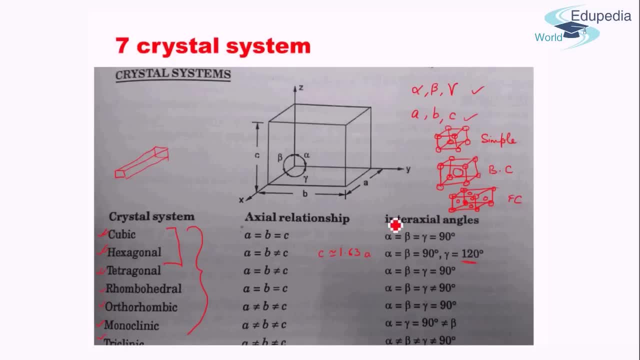 known as edge center, which does not exist in the cubic system. it does not exist in the cubic system, edge center, but in the system in which it does exist, the edge system- what will happen is something like this: this is not a cubic system. i'm not going to say what system supports. 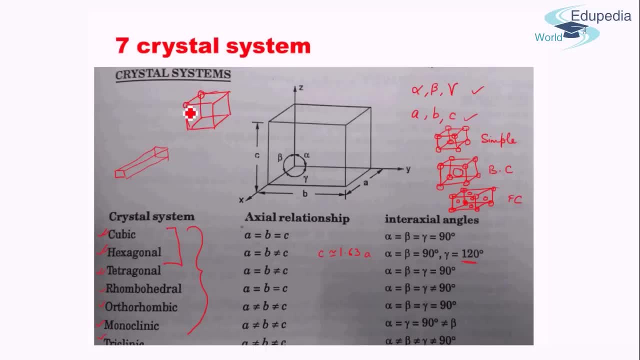 the edge center, its center system. but just know that there will be systems which will have edge center and in those system we will have eight atoms at the eight corners and two atoms, one at the top face and one at the bottom bottom face. this is edge center, right? so these are the four different.